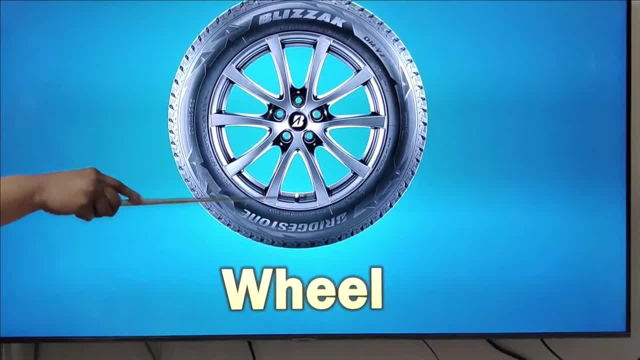 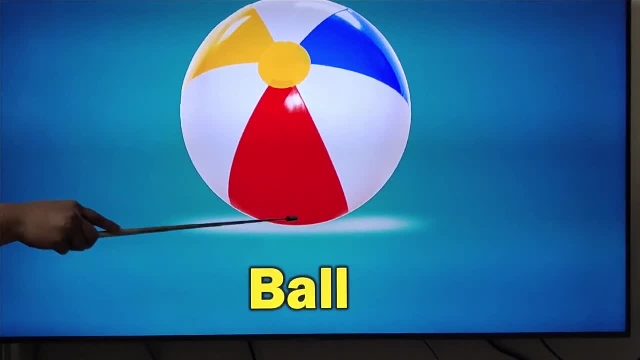 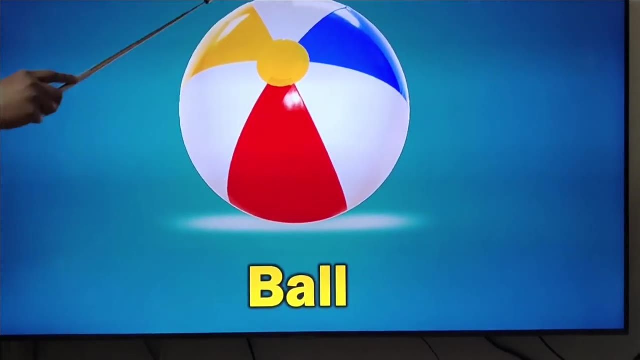 So wheel is an example for circle. Wheel is an example for circle Ball. b-a-l-l Ball Ball, also round in shape. Ball is round in shape and it has no corners. Ball is round in shape, It has no corners, So ball is an example for circle. 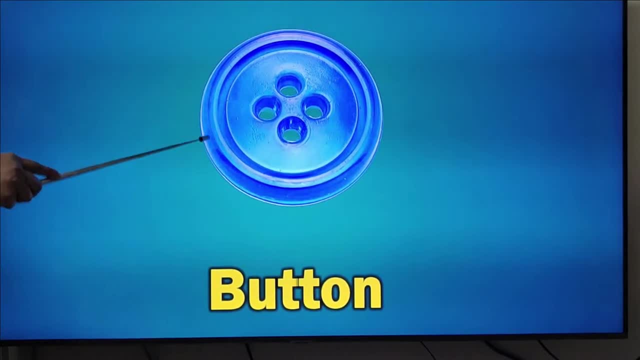 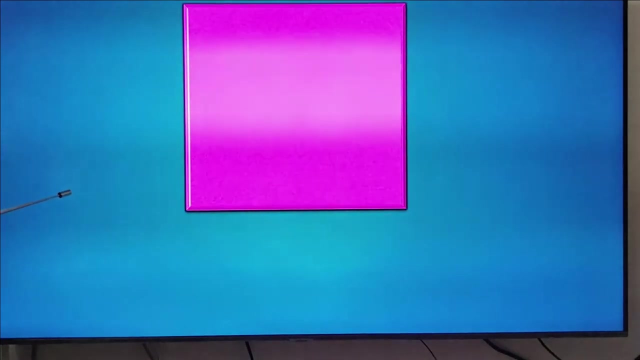 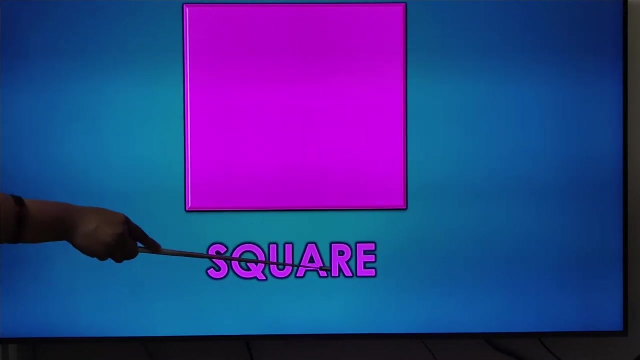 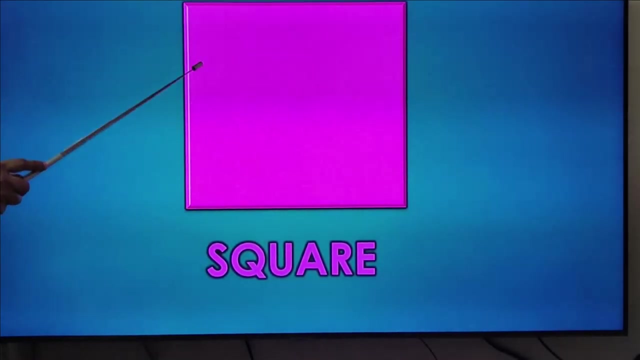 Button b-u-t-t-o-n Button. Button also round in shape. Button is round in shape. It has no corners. It is round in shape and it has no corners. So button is also an example for circle Square: S-q-u-a-r-e Square, S-q-u-a-r-e Square. A square has four sides. A square has four sides. 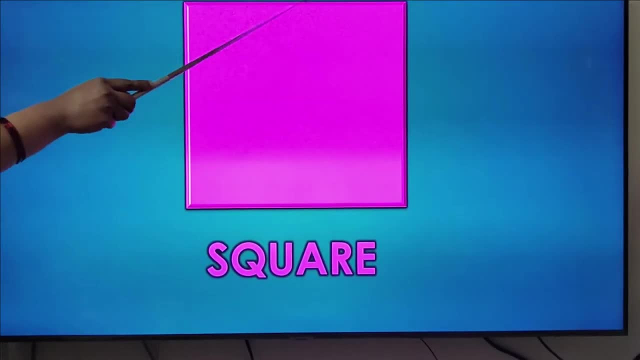 1,, 2,, 3,, 4.. A square has four sides and four corners: 1,, 2,, 3,, 4.. 1,, 2,, 3,, 4.. A square has four sides and four corners: children. 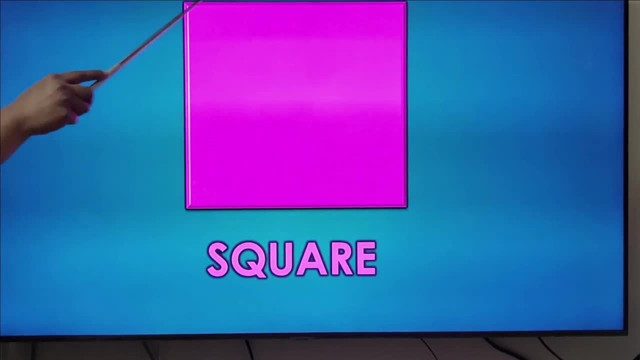 A square has how many sides. A square has four sides- 1,, 2,, 3,, 4 and 4 corners- And all the sides should be equal. All the sides for the square should be equal. All the four sides should be equal for square. 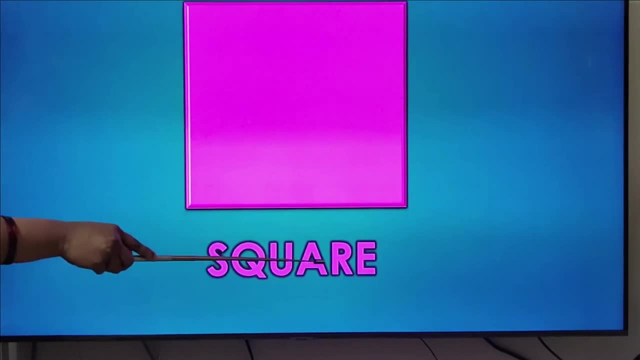 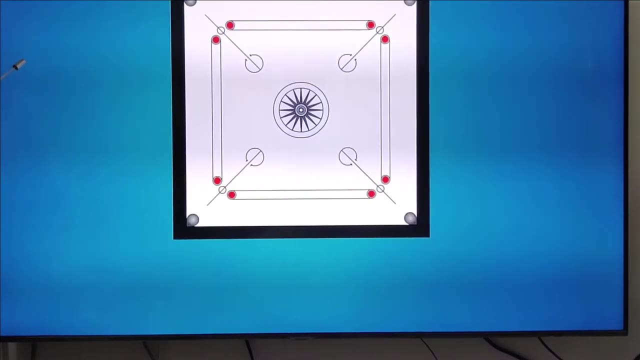 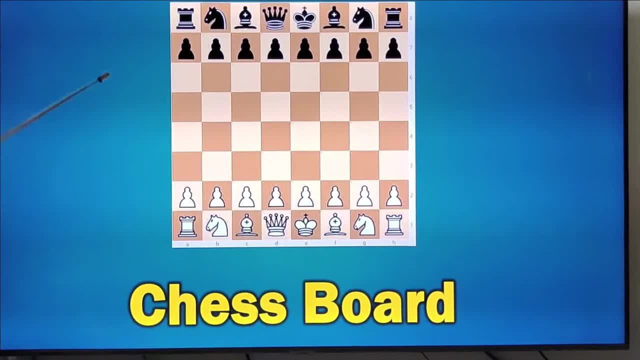 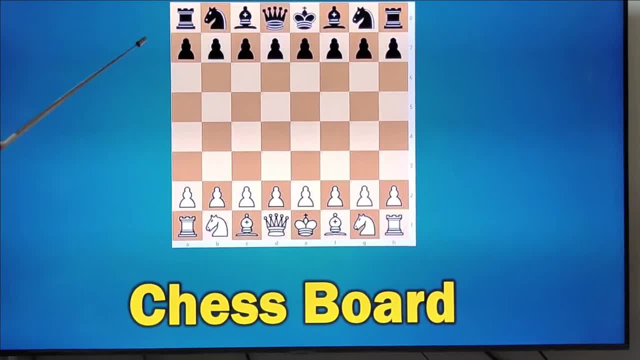 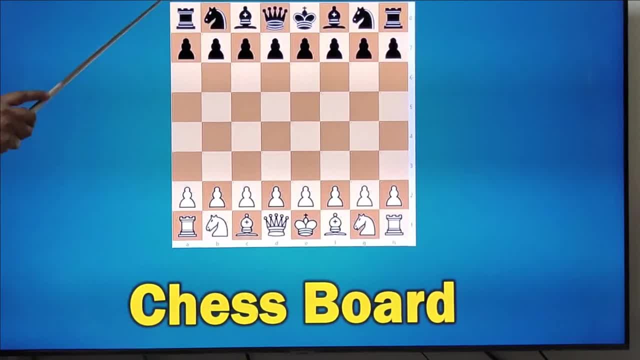 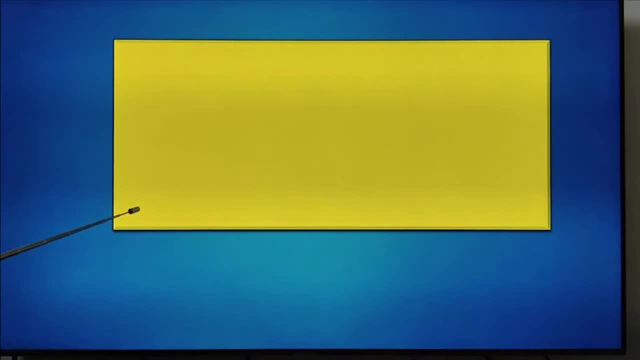 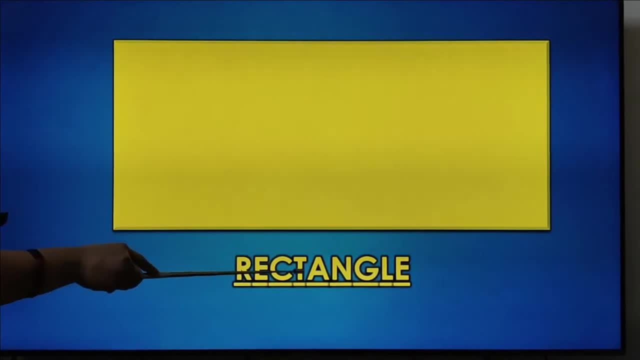 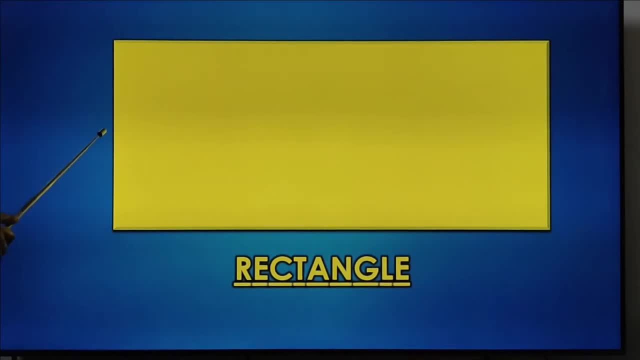 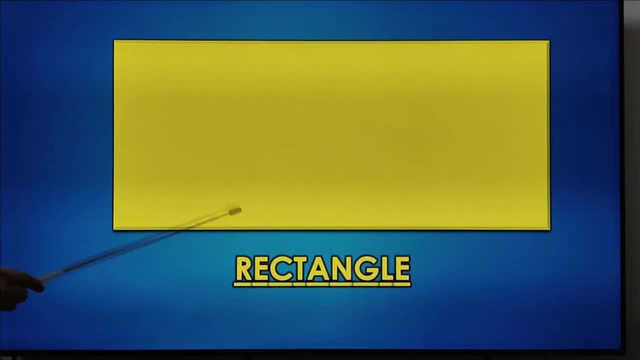 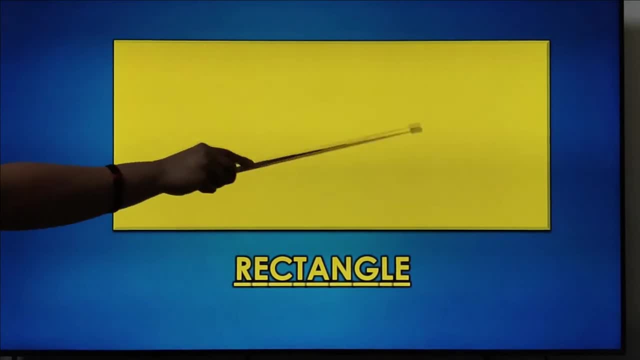 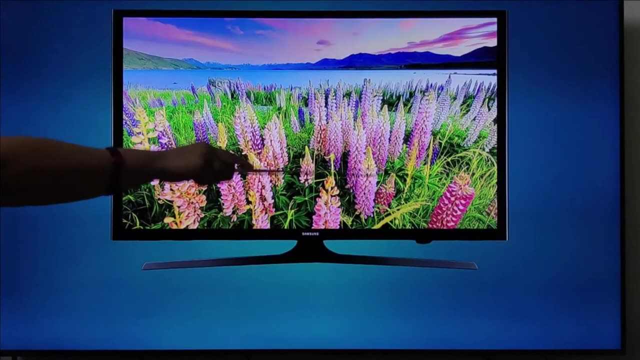 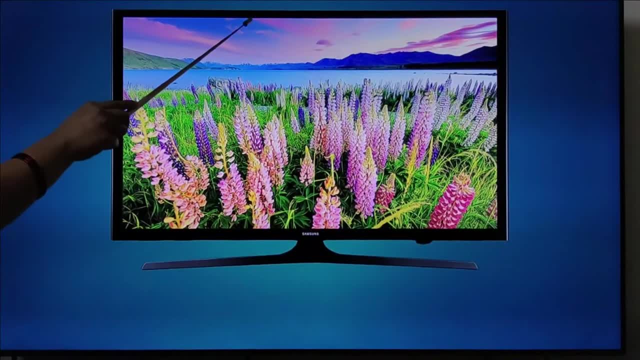 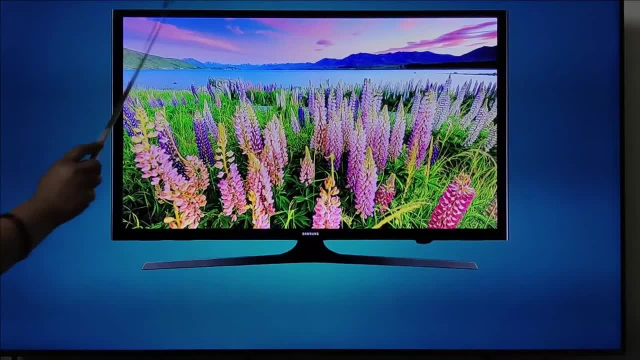 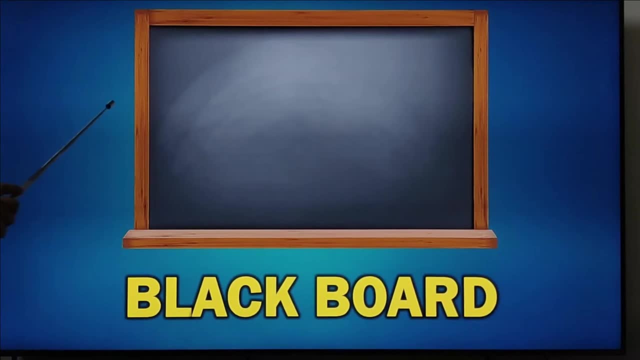 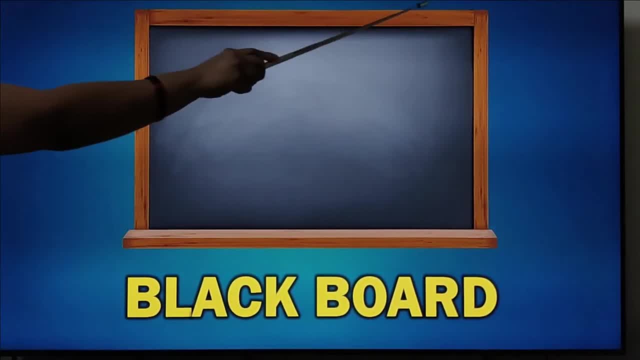 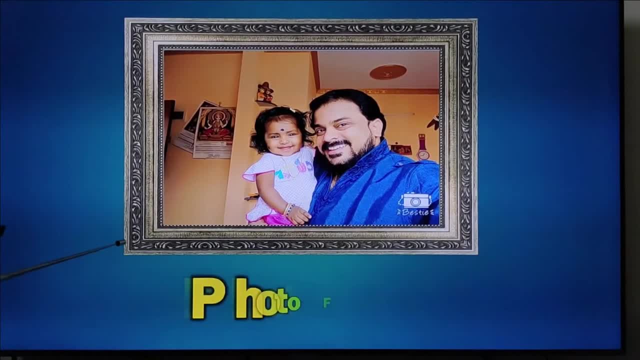 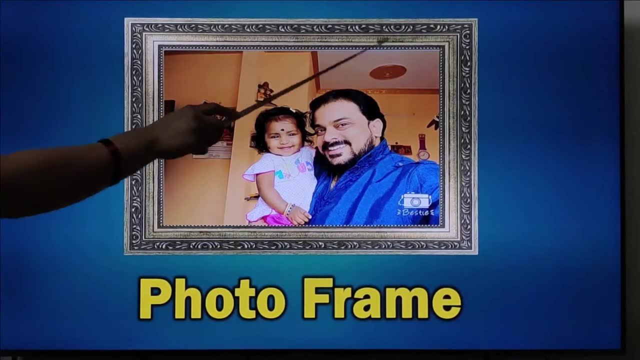 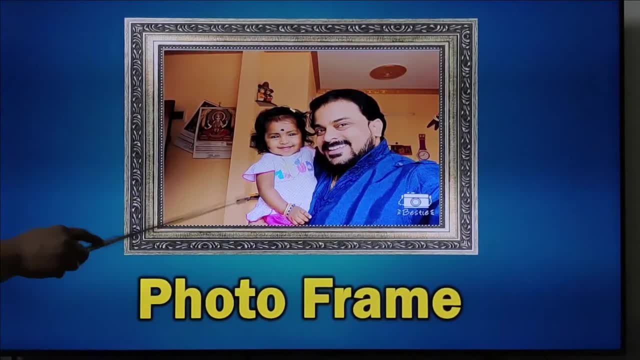 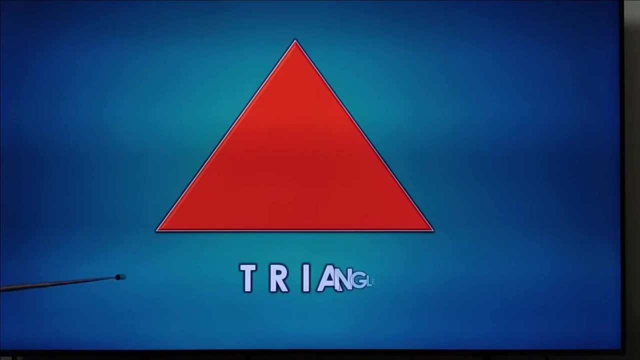 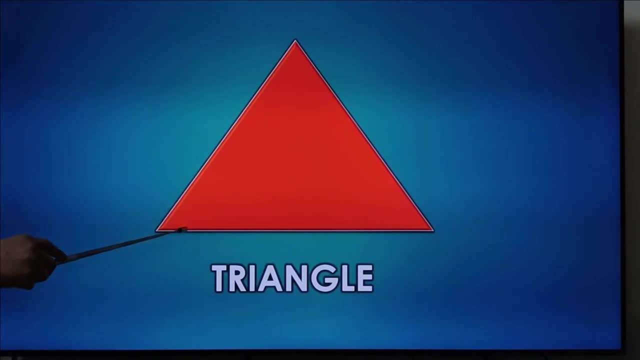 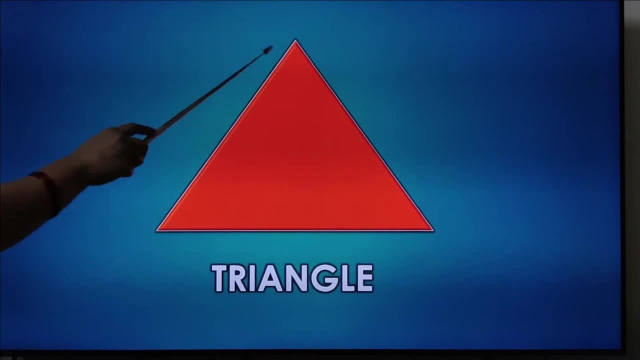 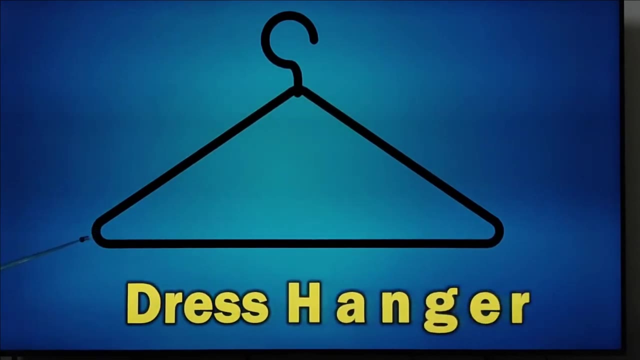 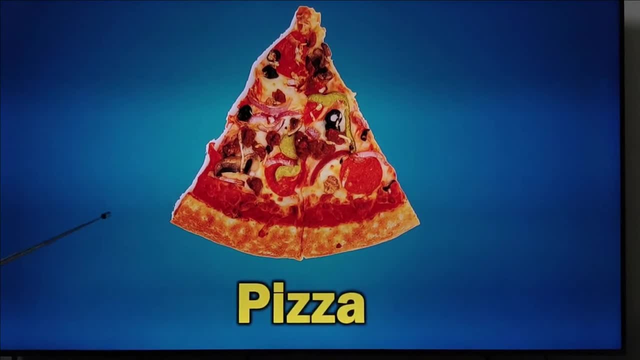 pizza, yummy pizza, this you know very well. piece of peas, this is a piece of pizza. this piece of is also an example of triangle. when you cut the pizza, if we get triangle shape- see listen here. when you cut the pizza, we get triangle shape, three sides and three corners: one, two, three. 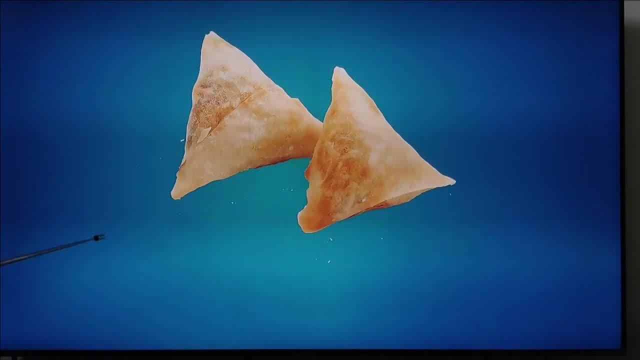 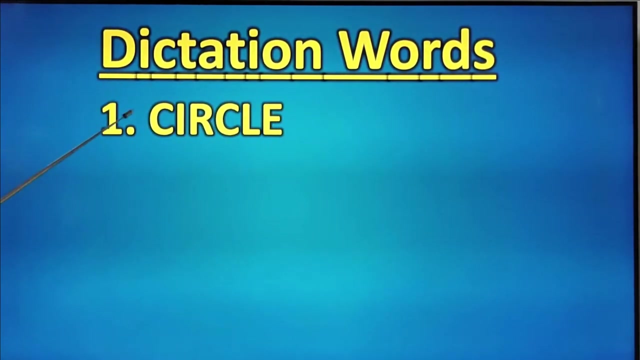 three corners and three sides, samosa. samosa also an example for triangle: three corners and three, three sides. it has three corners and three sides. so samosa also an example for triangle. dictation words number one: CIR CLE circle, CIR CLE circle, CIR CLE circle. repeat with me children: CIR CLE circle. 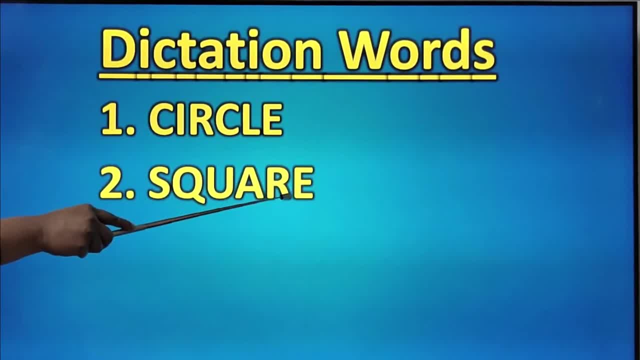 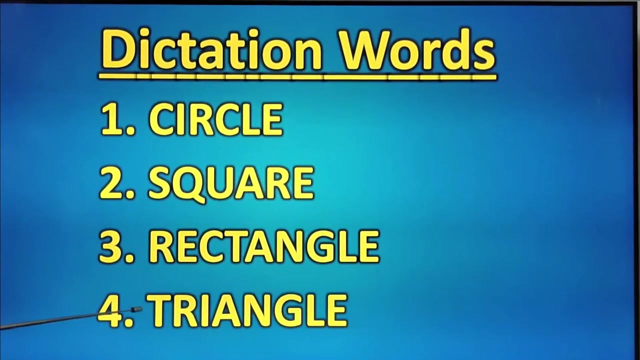 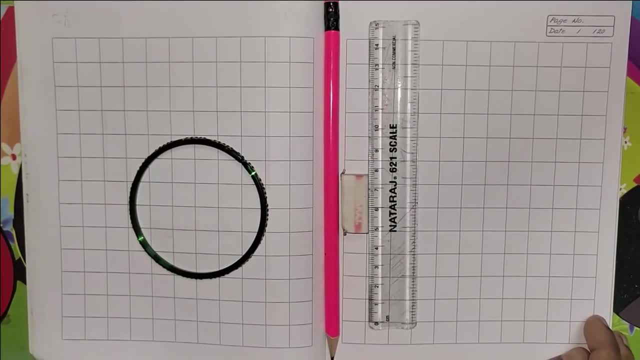 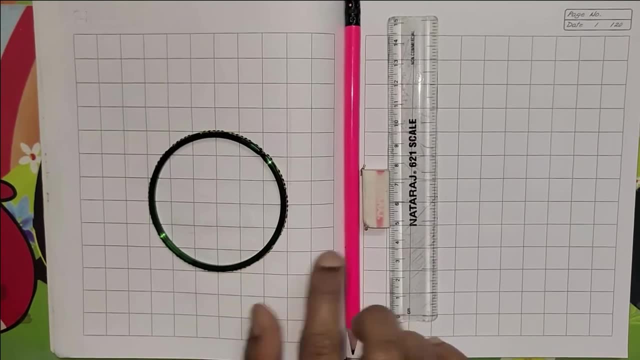 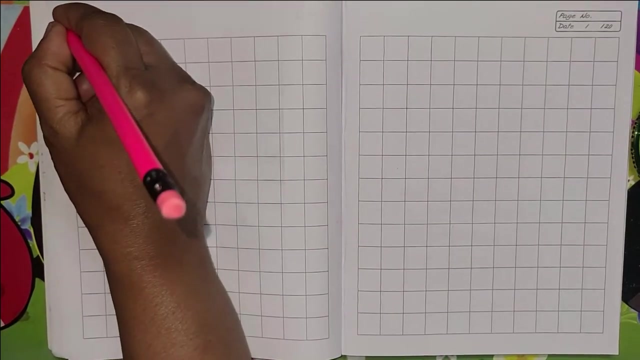 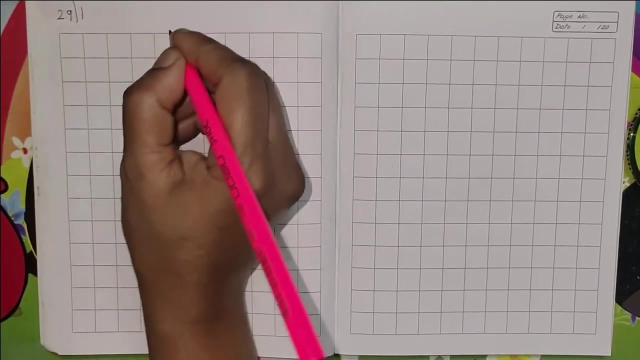 now let's see how to draw shapes in the notebook. first take one bangle pencil eraser and scale. take one bangle pencil, eraser and scale. first write the date 2929 bar 1. then write the heading in the first line: S, H, A, P E. 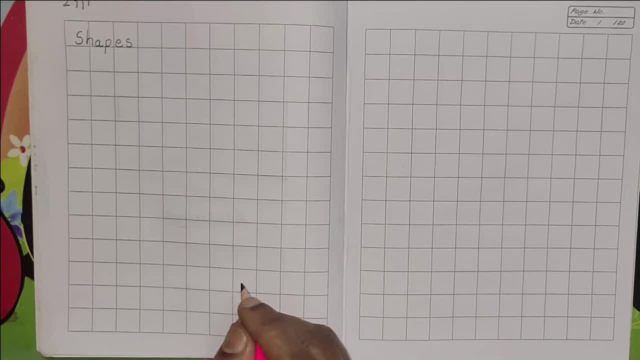 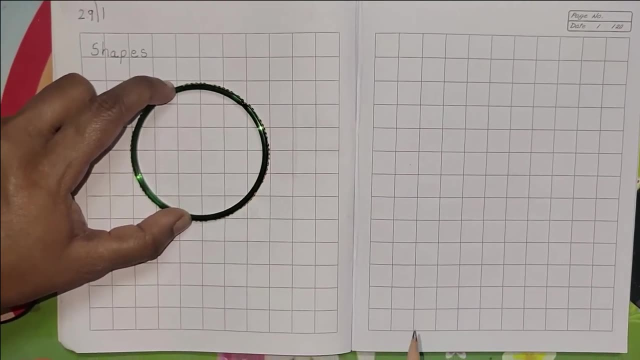 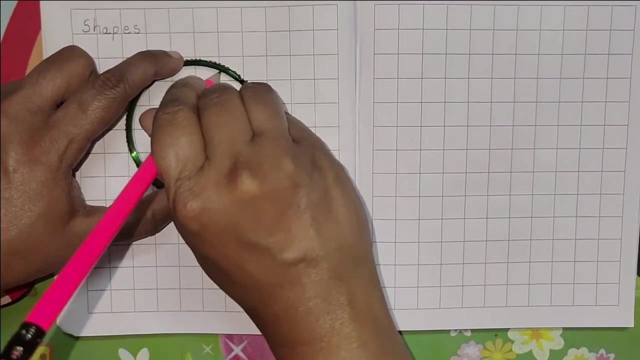 S H A P E, S, H A P E S shapes. first shape is circle. lets draw the circle. now. keep the bangle like this. children hold the bangle like this and draw circle inside the bangle. hold the bangle tightly and then draw circle like this. take the bangle. 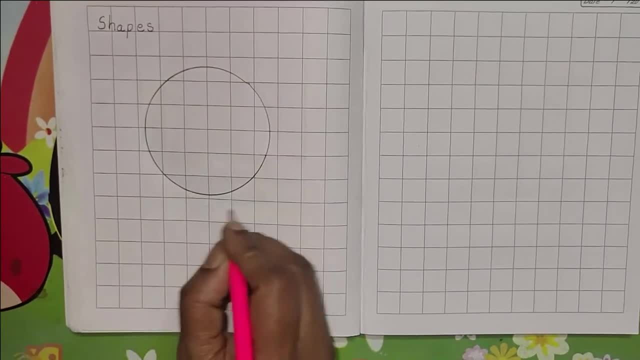 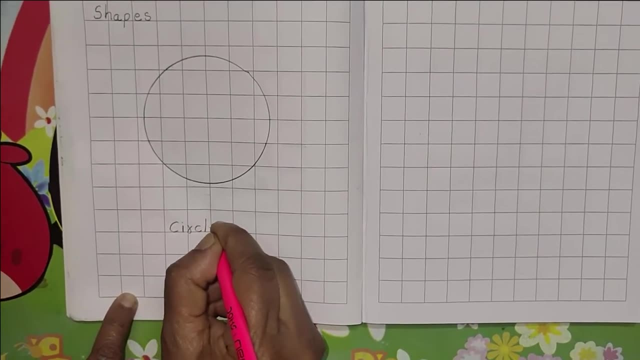 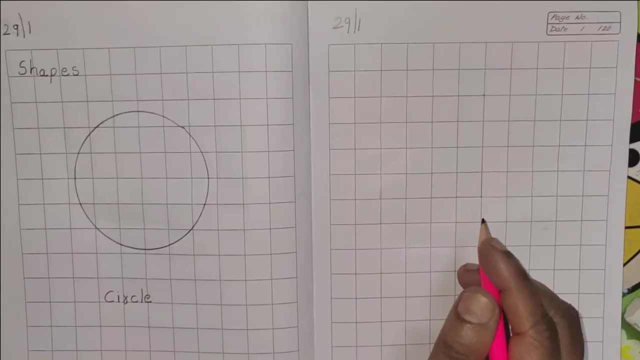 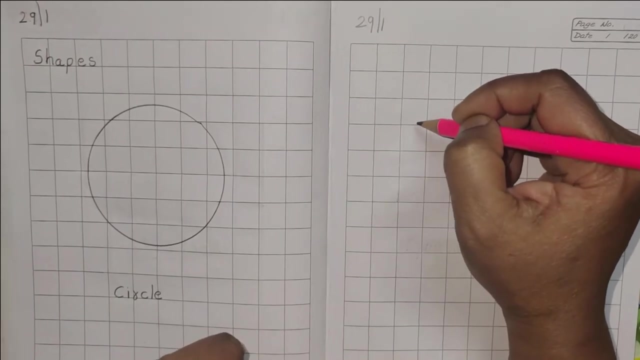 see, we got this circle shape now. now write the spelling down to that: C? I R or c? l e circle: c? i or c? l e circle now next. now let's draw square. first leave three lines from up: children: one, two, three. then leave three boxes from your left side free. leave three boxes. 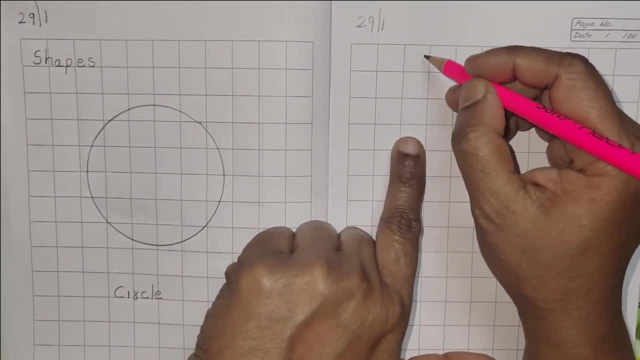 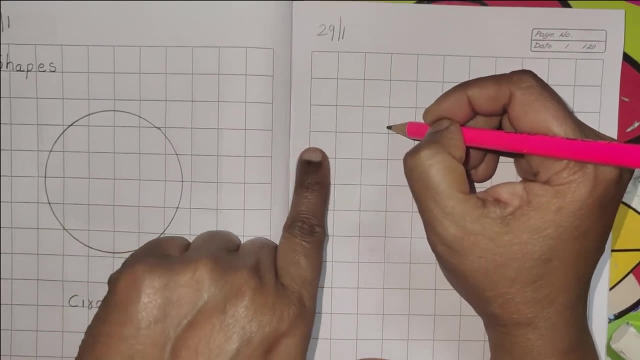 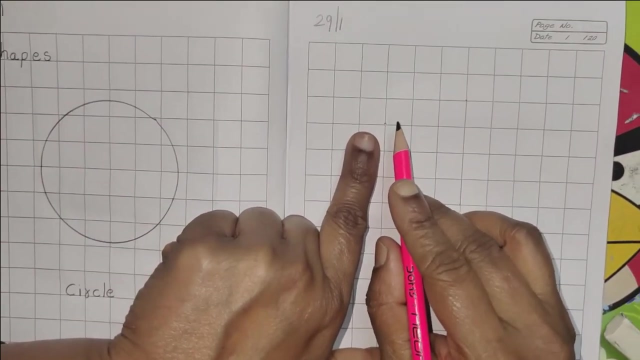 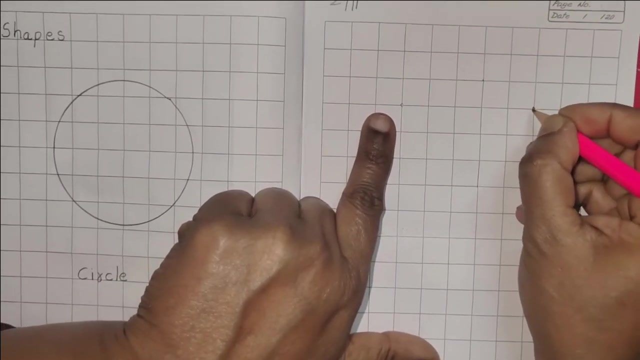 from your left side: one, two, three, three lines from up and three, three boxes from up and three boxes from your left side. one, two, three, one, two, three. keep one dot now count for five boxes. one, two, three, four, five. keep one dot in the fifth box. keep one dot in the fifth box. 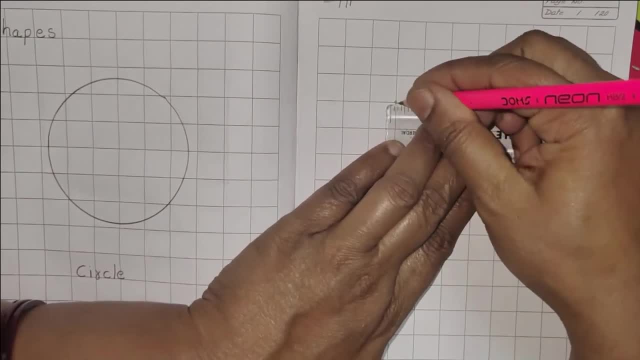 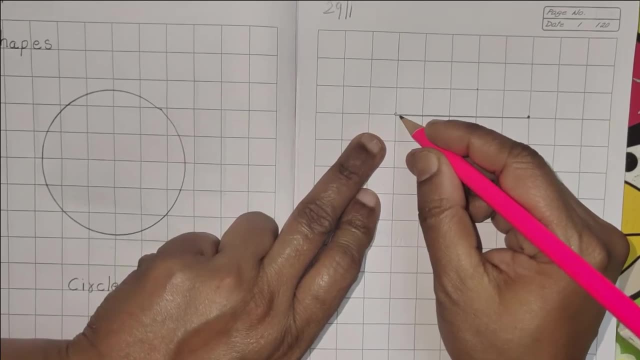 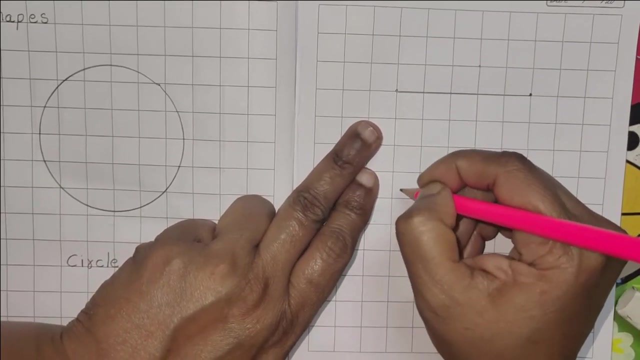 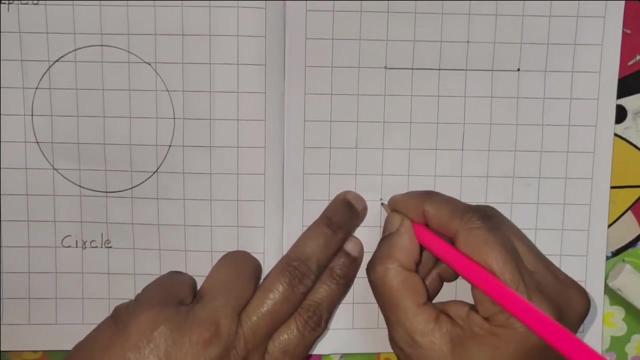 and join the two dots. draw one sleeping line. join the two two dots, then down to the line. count again five boxes. down to that line, count five boxes: one, two, three, four, five. count five boxes: one, two, three, four, five. keep one dot in the fifth box. keep one dot in the fifth box. 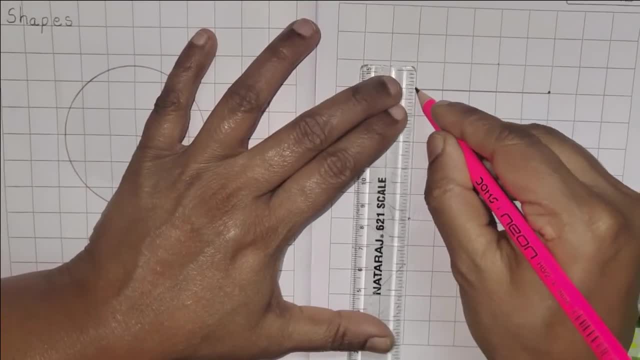 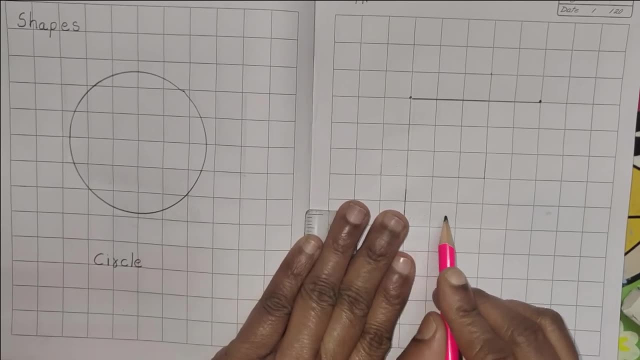 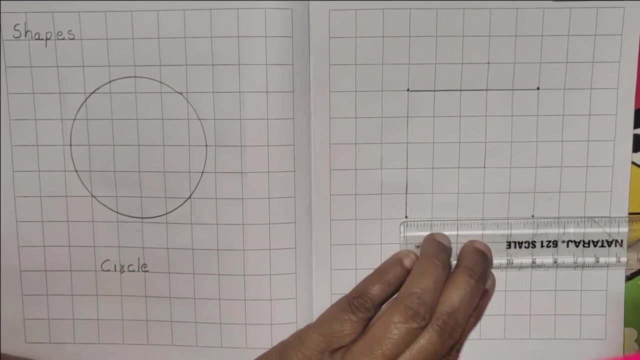 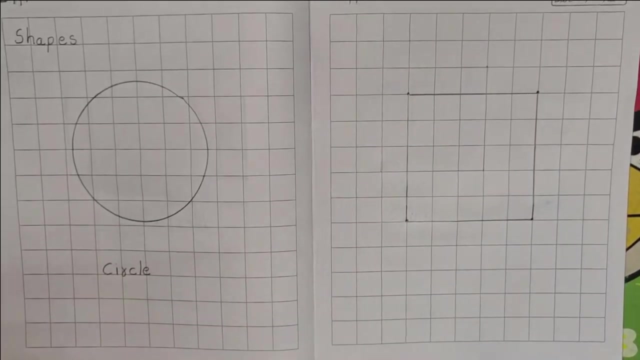 now join the two dots. now again count five boxes from your left side, five boxes from your left side. one, two, three, four, five. keep one dot in the fifth box. now join the dots. now we got the square for square. all the four sides should be equal for. 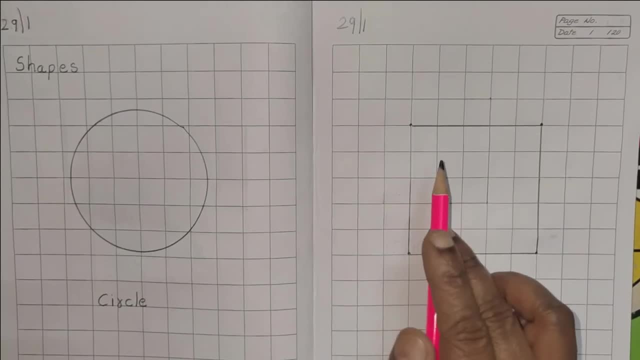 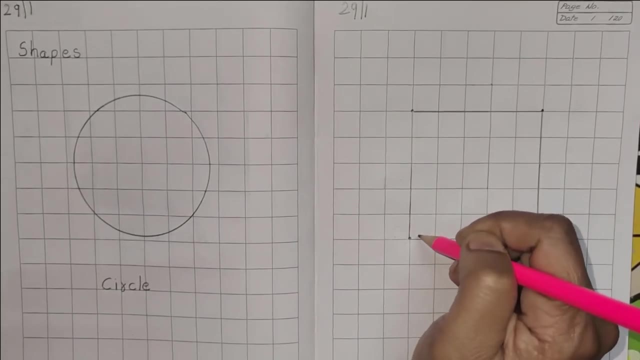 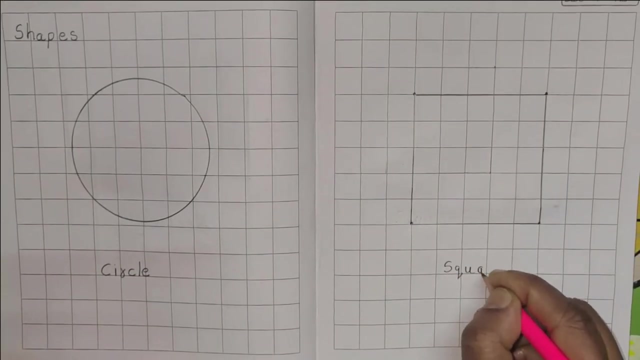 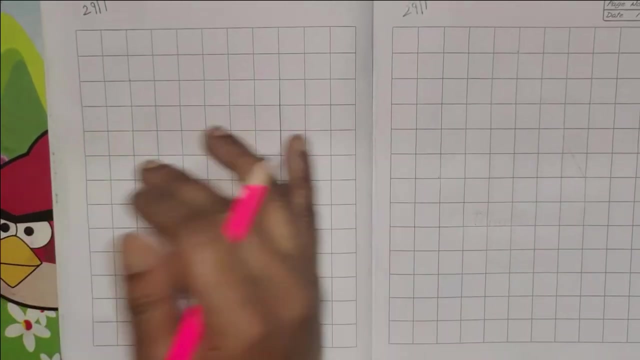 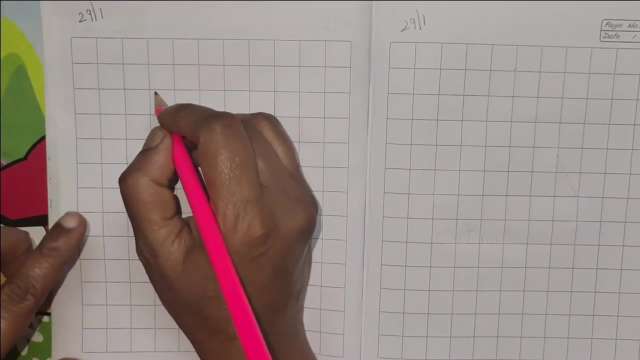 square. all the four sides should be equal. now count the boxes: one, two, three, four, five. yes, it is equal here. one, two, three, four, five. yes, it is equal. now let's write the spelling square. Now let's draw rectangle For rectangle. also same way. leave three lines from up and 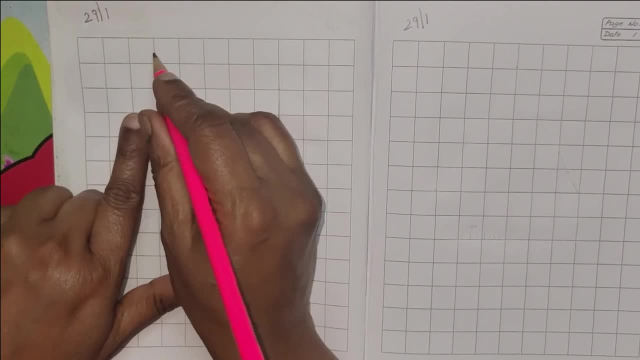 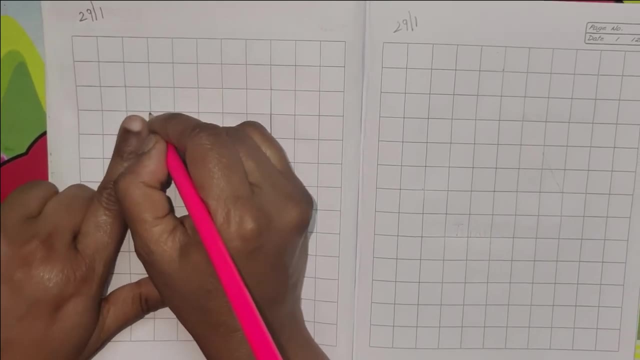 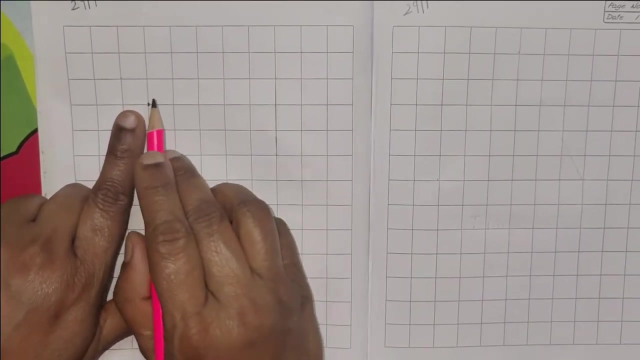 leave three lines from your left side, Leave three lines from up, three boxes from up and leave three boxes from the left side, One, two, three, and one two, three. Keep the dot in the third box. Keep the dot in the third box. Then count five boxes: One, two, three, four, five. 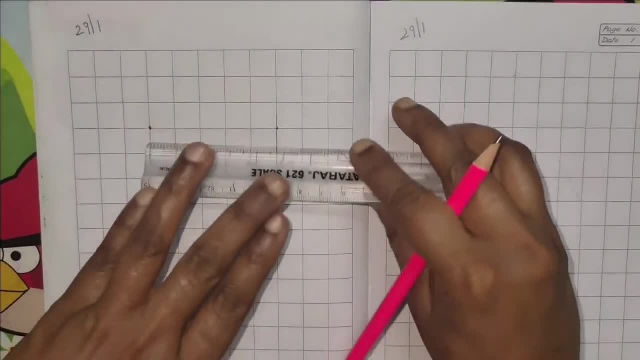 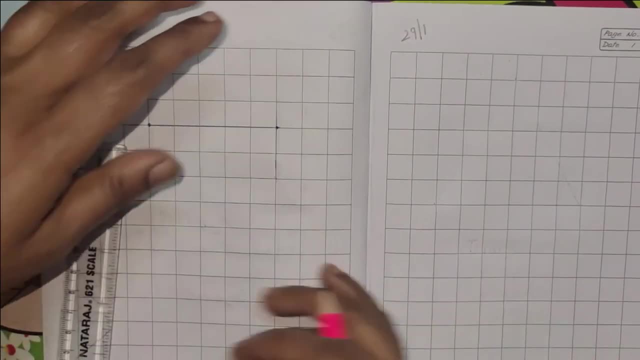 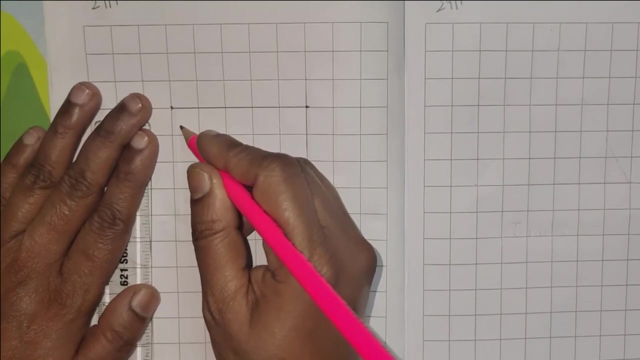 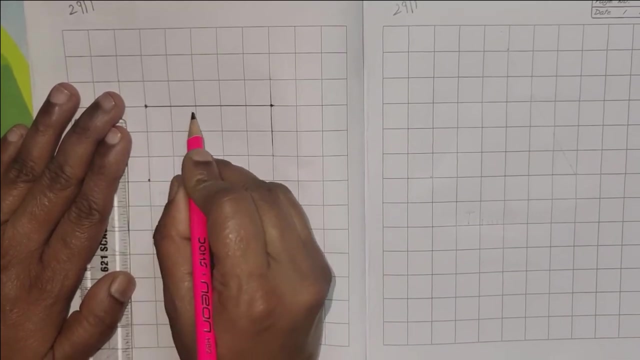 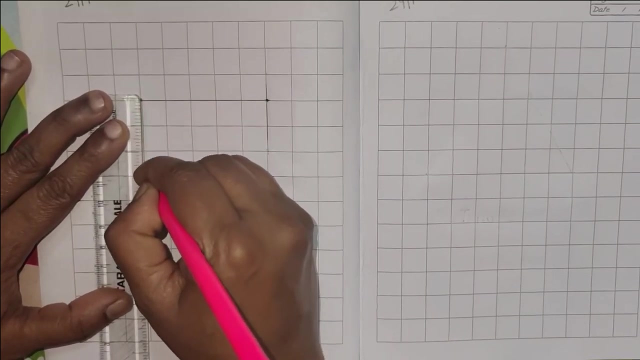 Keep the dot in the fifth box. Then join the dots. Same way as square, But for rectangle, two opposite sides. So down you should count only three boxes: One, two, three. Keep one dot Next to the line. count three boxes Next to the line. count three boxes: One, two, three and keep one dot. Join the dots. 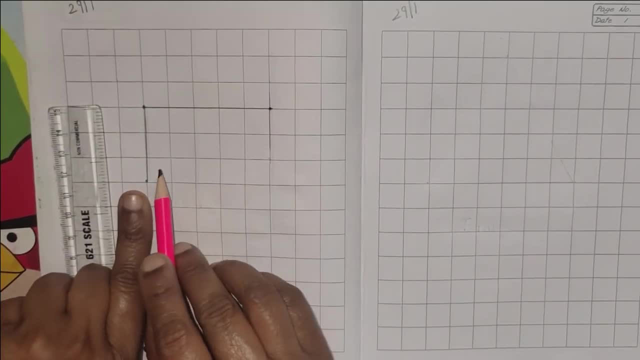 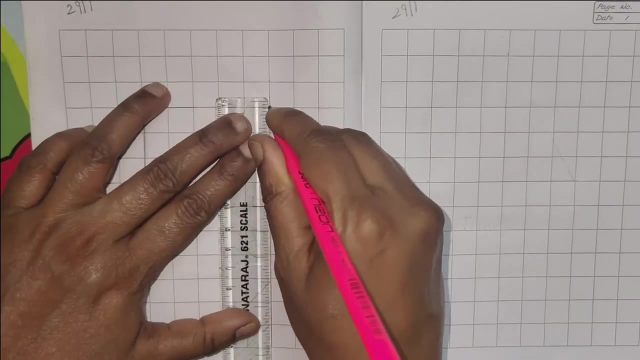 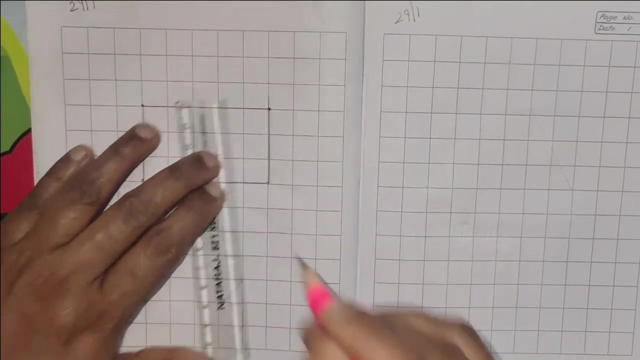 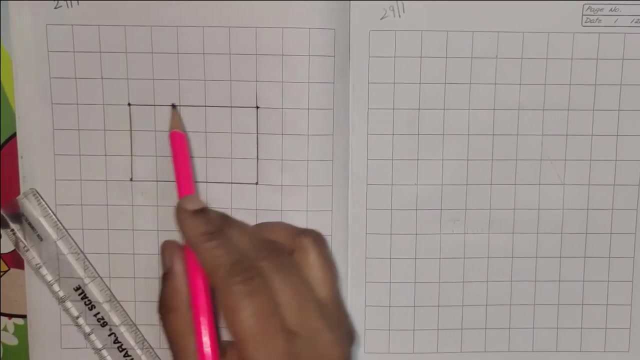 Now, from your left side, Now from your left side, count five boxes: One, two, three, four, five. Keep one dot And join the dots. Now join all the dots. Now listen here, children. Two opposite sides are equal for rectangle One, two, three, four, five. So two opposite sleeping lines are equal for. 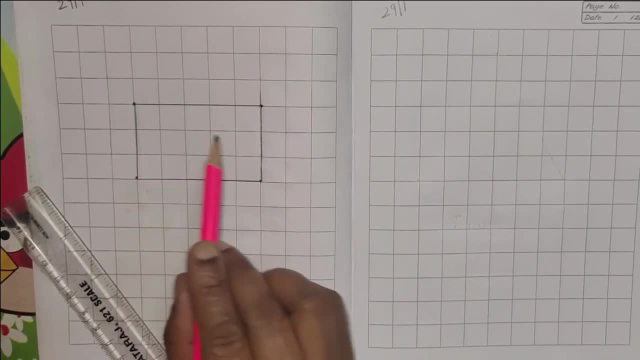 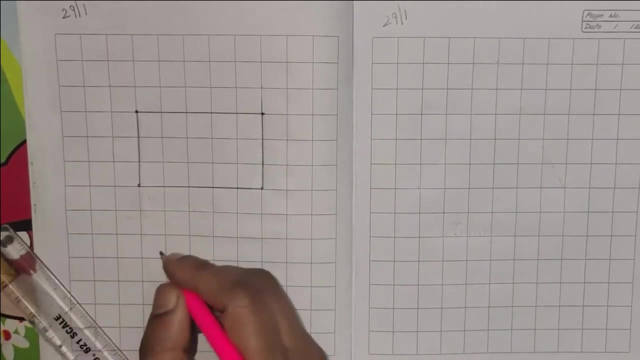 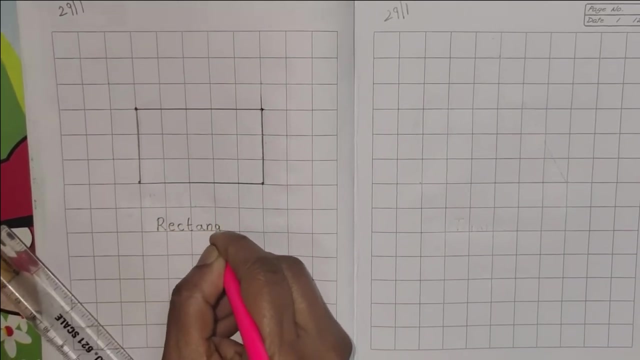 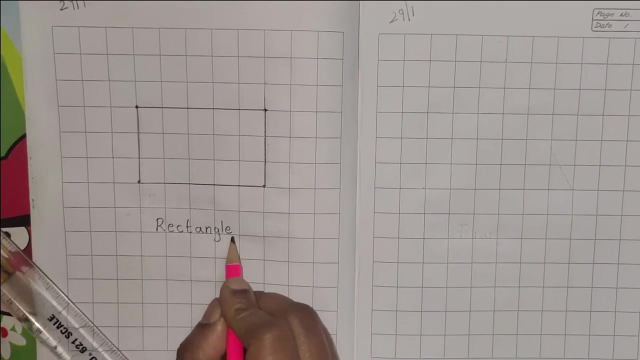 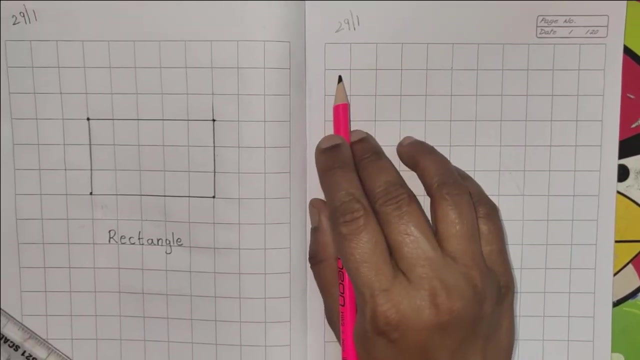 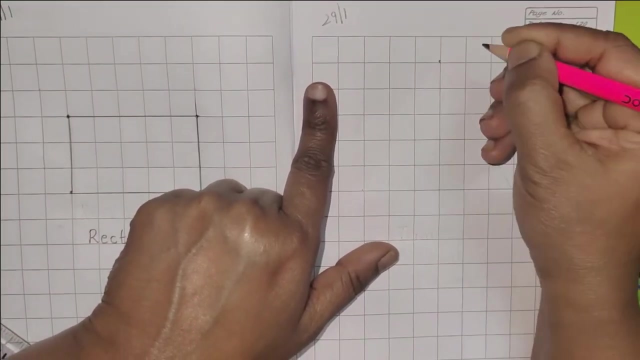 rectangles. This side rectangle and two opposite standing line are equal for rectangle. Two opposite sides are equal for rectangle. Let's write the spelling R-E-C-T-A-N-G-L-E rectangle. R-E-C-T-A-N-G-L-E rectangle, R-E-C-T-A-N-G-L-E rectangle. Now let's draw triangle For triangle. count five boxes from your left side: One, two, three, four, five. Keep one dot in the fifth box. 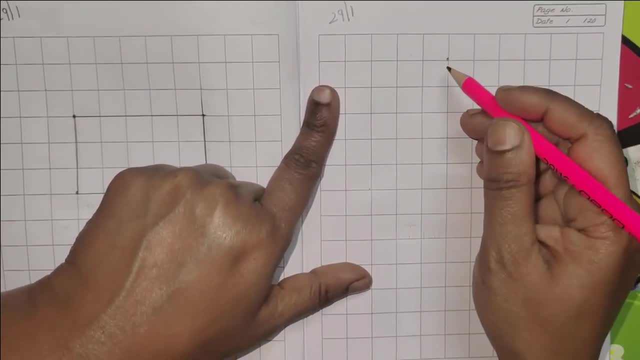 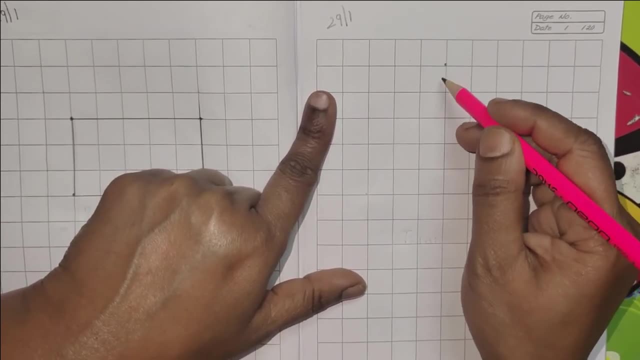 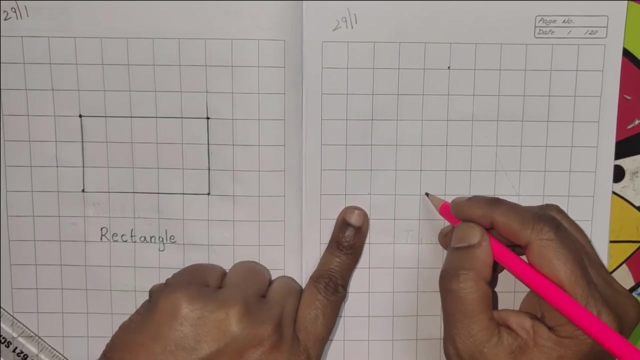 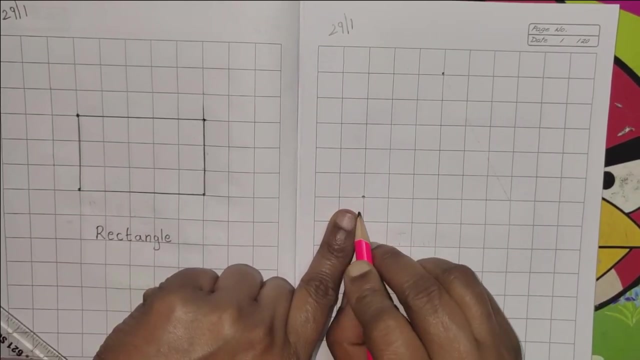 Keep one dot in the fifth box. Then again count five boxes from that down to that dot. Count five boxes down to that dot. One, two, three, four, five. After counting from your left side, leave two boxes. Leave two boxes from your left side and keep one dot. Leave two boxes from your left side and keep one dot. 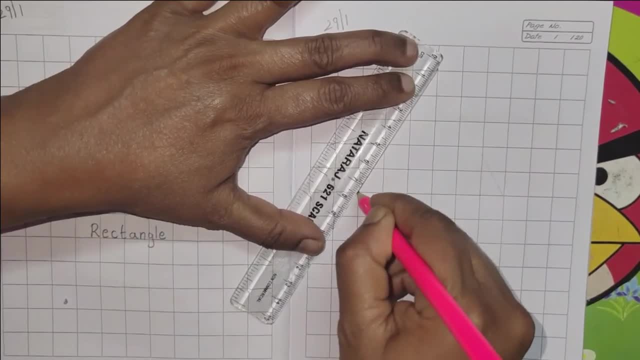 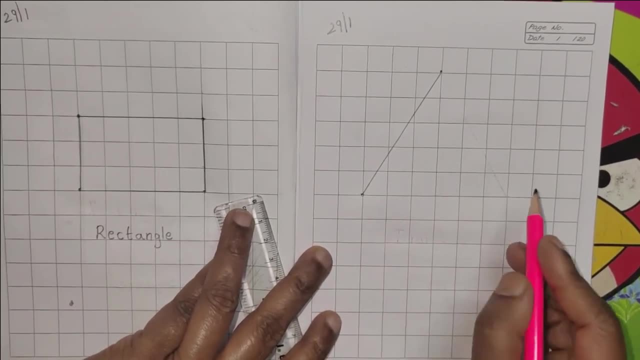 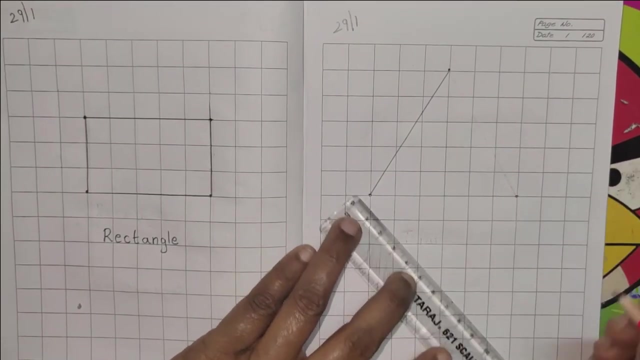 Then draw one slanting line. Then draw one slanting line. Join the dots. Then again count five boxes from the dot One, two, three, four, five. One, two, three, four, five. Keep one dot in the fifth box. Join the dots. 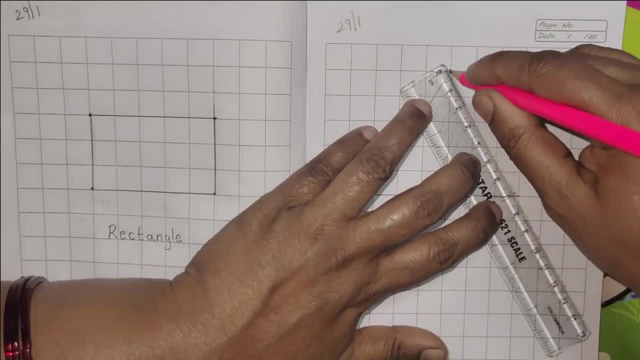 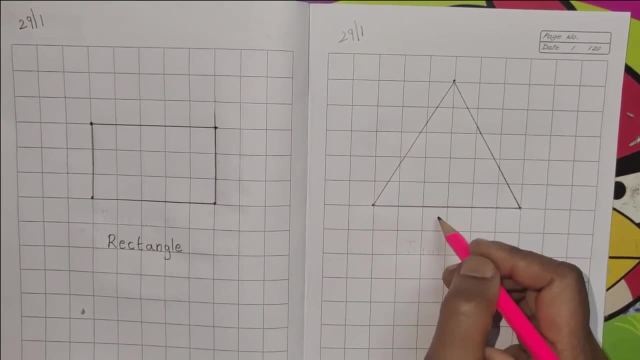 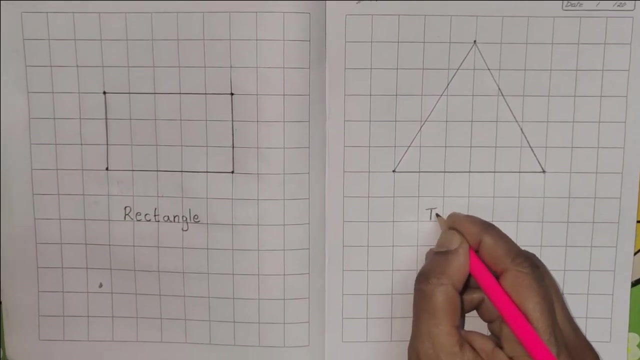 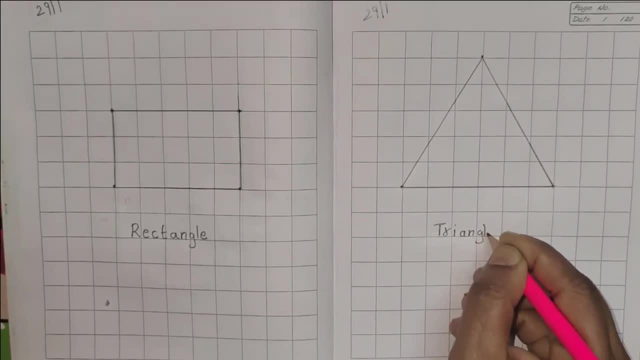 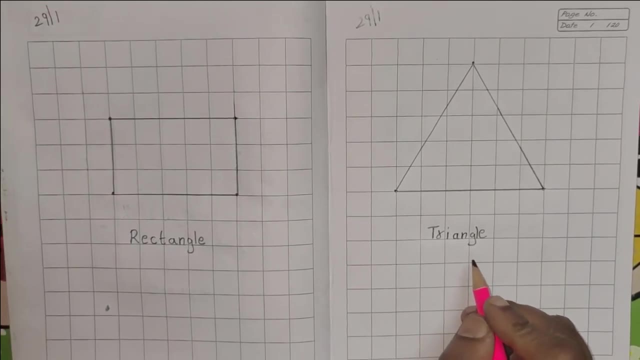 T-R-I-A-N-G-L-E triangle. T-R-I-A-N-G-L-E triangle- T-R-I-A-N-G-L-E triangle- Parents, please guide the children to draw the shapes. Thank you.